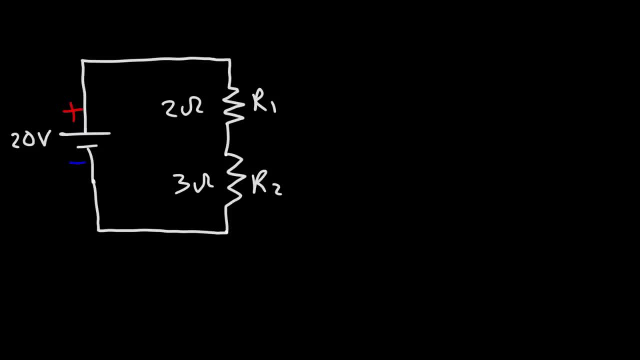 the voltage drop across R1 and what is the voltage drop across R2?? So what do you think we can do to find the answer? In order to calculate the voltage drop across a resistor, you need to know the resistance and the current flowing through the resistor. So first we 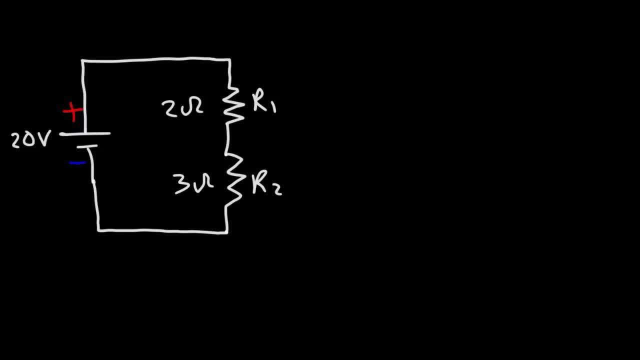 need to calculate the current flowing in the circuit. So how can we do that? Well, first we need to know what type of circuit we have, and this is a series circuit. The reason why it's called a series circuit is because the current has only one path to flow through. 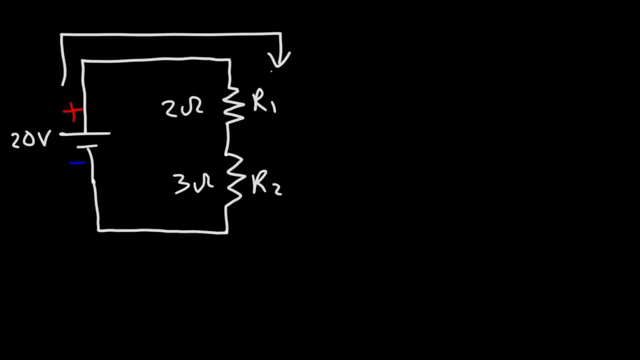 these resistors. So these resistors are in series. Now. in a parallel circuit the current can flow in multiple directions. When there's multiple paths for the current to flow, then you have a parallel circuit. But in a series circuit there's only one path for the current. 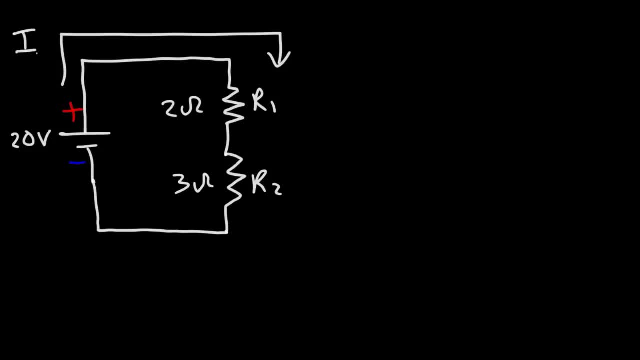 to flow. Now, the current that we're dealing with is conventional current, where it flows from the positive terminal to the negative terminal. But keep in mind that electrons, they flow in the opposite direction, From the negative terminal of the battery to the positive terminal. Now, before we can calculate the current in a circuit, we need to determine: 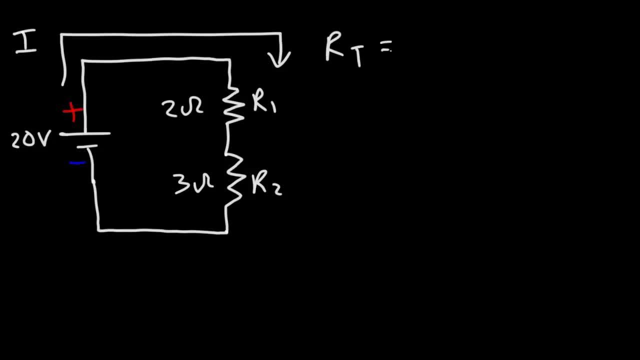 the total resistance. So let's go ahead and calculate the current in a series circuit For resistors. in series, the total resistance is the sum of all the resistors. So in this example it's simply 2 plus 3, which is 5 ohms. So that's the total resistance of this. 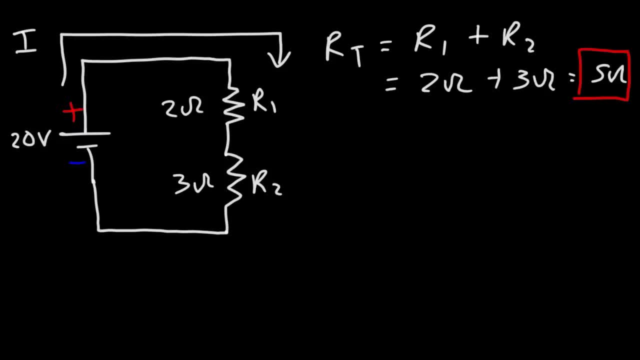 circuit. Now to calculate the current flowing in a circuit, we're going to use the voltage of the battery and the current flowing in a circuit times the total resistance. So this comes from Ohm's law, And V equals IR, So the voltage of the battery is 20.. The total resistance is 5. 20 divided. 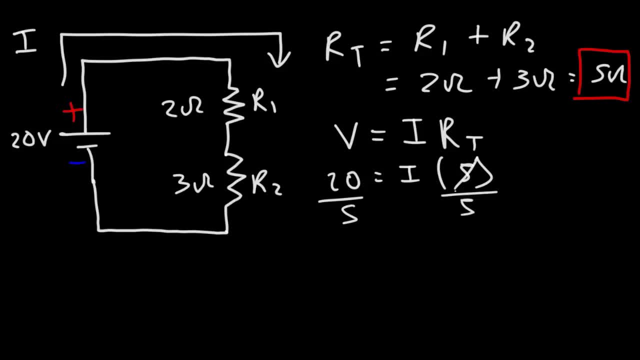 by 5 is 4.. So the current flowing in the circuit is 4 amps. Now, once we have the current, we can now calculate the voltage drop across each resistor: ghosted silence. Now we're going to use Ohm's Law again: at V equals IR, But the voltage across the resistance 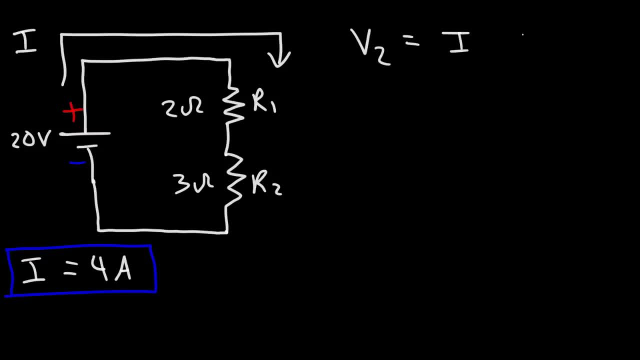 resistor 2 is going to be the current that's flowing in a circuit times resistor 2.. So we have a current of 4 amps times a resistance of 3 ohms, so that gives us a voltage drop of 12.. Now V1 is going to be I times R1, so that's a current of 4 amps times a resistance of 2 ohms, which is 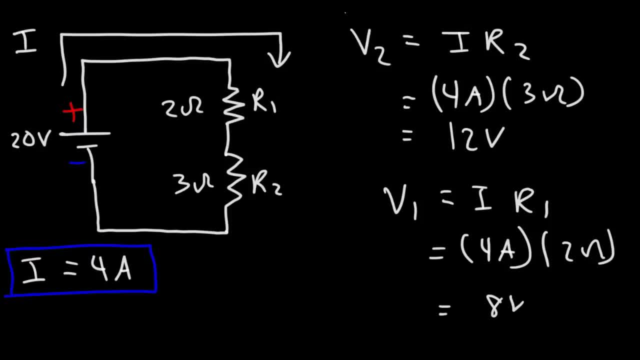 8 volts. So let's talk about what this means. If you were to take a voltmeter and connect it across R1, if you do it properly, you're going to get a voltage of 8 volts. If you do so across R2, you're. 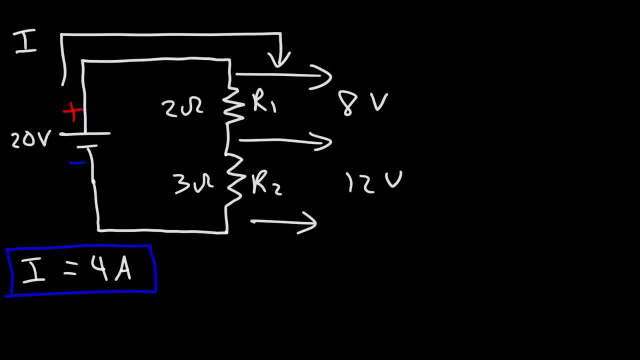 going to get a voltage of 12 volts. Notice that the sum of the voltage drops in this circuit is equivalent to the voltage of the battery, and it should be that way according to Kirchhoff's voltage law. If you want to get a voltage drop of 12 volts, you're going to need a voltage drop of 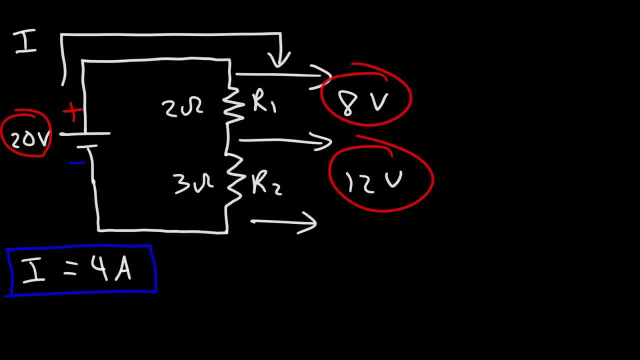 12 volts, which states that the sum of the voltages around a closed loop must add to 0.. Now the battery delivers energy to the circuit, so we're going to give it a positive voltage, and the resistors: they take away energy. they consume energy from the circuit, so we'll give it a negative voltage. thus, 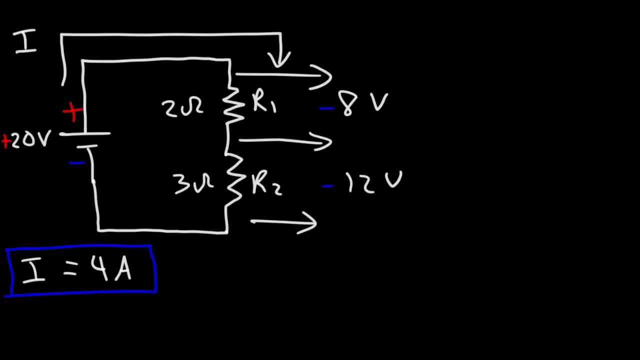 they're called voltage drops. So if you add positive 20 with negative 12 and negative 8, you're going to get 0.. So that's how you can calculate the voltage drop of a circuit. But for the sake of practice let's try another example. So this time there's going to be three. 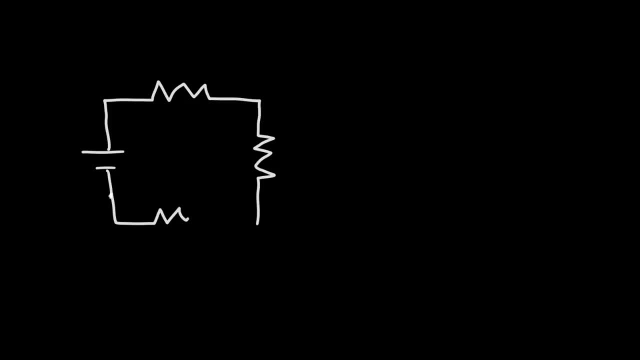 resistors instead of two. So we're going to call this R1, R2, and R3.. Now the voltage of the battery is going to be 36 volts in this case, and R1 is going to have a value of 5 ohms. R2 is going to be 4 ohms. R3 is going to be 3 ohms. So go ahead and take a minute and 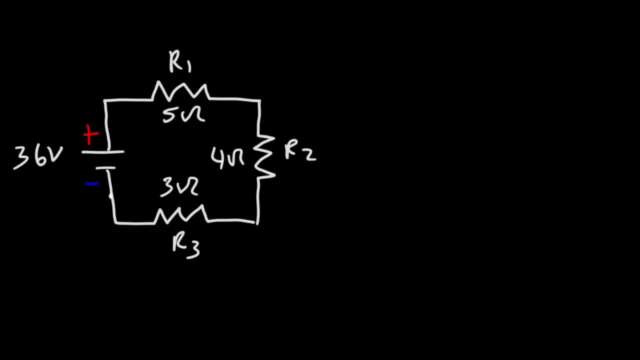 work on this example: Calculate the voltage drop across each resistor. Feel free to pause the video and try this problem. So let's begin by calculating the total resistance. So R1 plus R2 plus R3, so that's going to be 5 plus 4 plus 3.. 5 plus 4 is 9.. 9 plus 3 is 12.. So the total resistance in 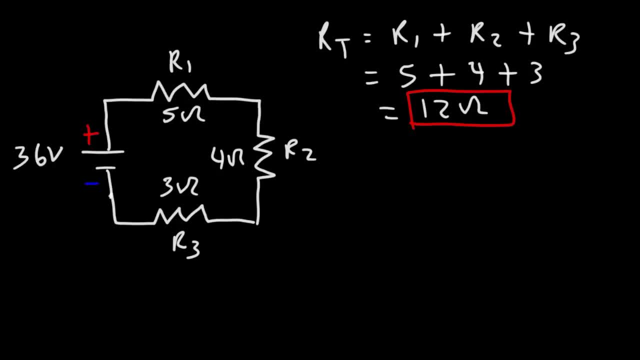 this circuit is 12 ohms. Step 2 is to calculate the current in a circuit. So, because it's only 1 ohm, we're going to calculate the current in a circuit. So, because it's only 1 ohm, we're going to. 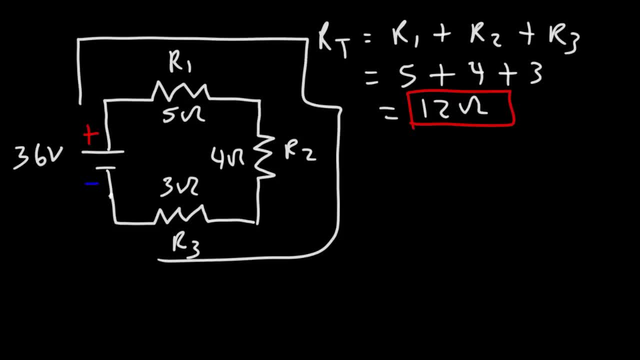 1 path for the current to flow. All three of these resistors are in series. The current is going to be the voltage of the battery divided by the total resistance of all the resistors in series. So the voltage is 36 volts, The total resistance is 12 ohms. So 36 divided by 12, that's going to give. 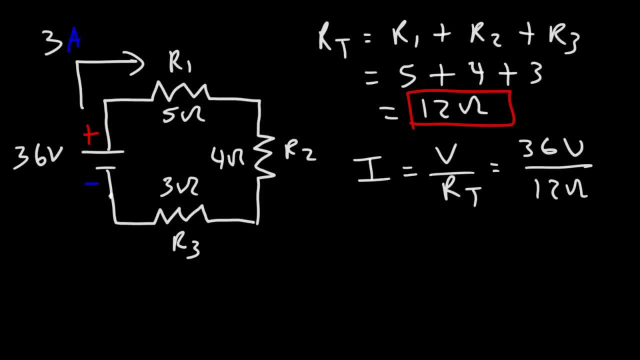 us a current of 3 amps. So now that we have the current in a circuit, we can now calculate the voltage drop across each resistor. So let's start with V1.. V1 is going to be the current times R1. So that's a current of 3 amps times a resistance of 5 ohms. So that gives us a voltage drop of 15 volts. 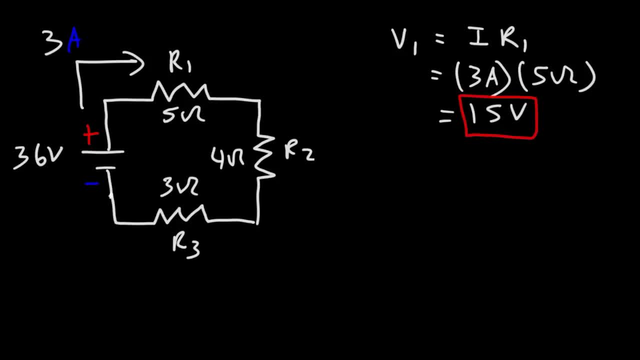 Now let's move on to V2.. The voltage drop across R2 is going to be I times R2.. So that's going to give. So that's a current of 3 amps times 4 ohms. so that gives us a voltage of 12 volts. 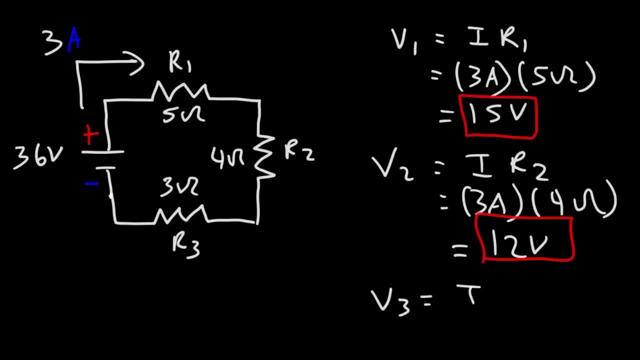 And now to calculate the voltage drop across R3, it's going to be I times R3, so 3 times resistance of 3, which is going to give us 9 volts. So now let's add these three numbers: 15,, 12, and 9.. 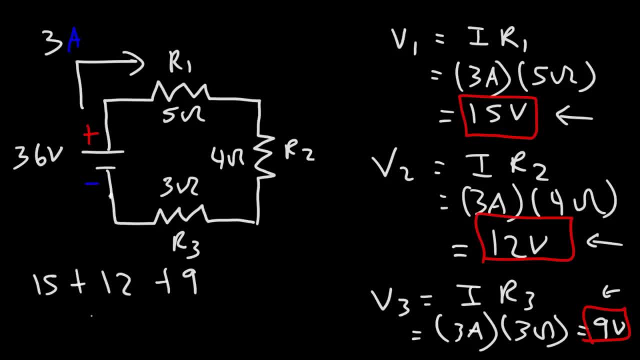 So 15 plus 12, that's 27,, 27 plus 9 is 36, and that's a quick way to tell if you performed this problem correctly. So these are the voltage drops of each resistor. that's how you can find them. 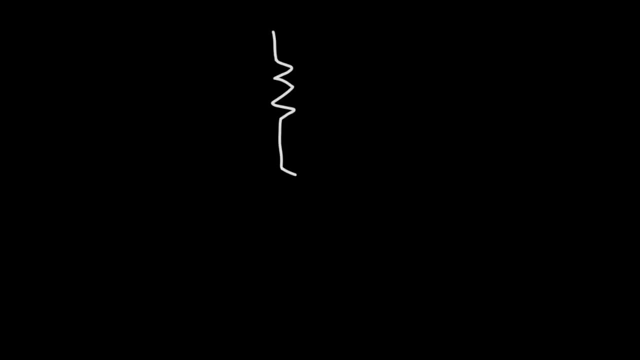 Now let's work on a different type of problem. So let's say we have these two resistors and three points of interest. We're going to call this point A, point B and point C And let's say R1 has a resistance of 8 ohms and R2 has a resistance of, let's say, 15 ohms. 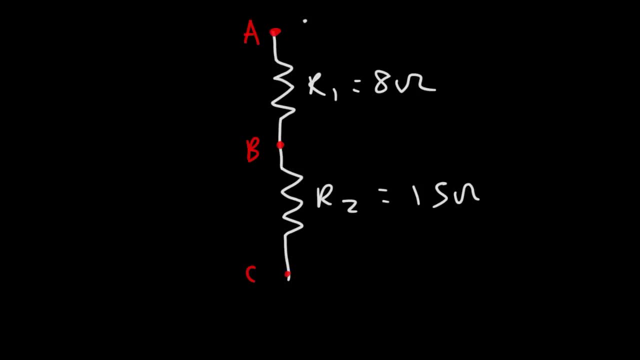 Now let's say the potential at point A is 50 volts And the potential at point B is 10 volts. What is the voltage drop across R2? And what is the electric potential at point C? Feel free to pause the video and try this problem. 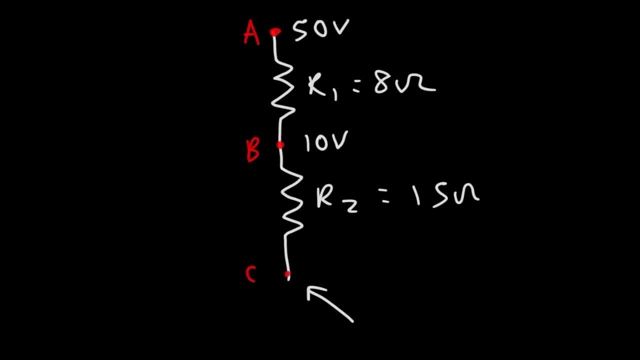 Now, what do you think is the first thing that we should do? The first thing we need to do is calculate the voltage drop across R1.. The voltage drop across R1 is the difference Between the electric potential at point A and point B. 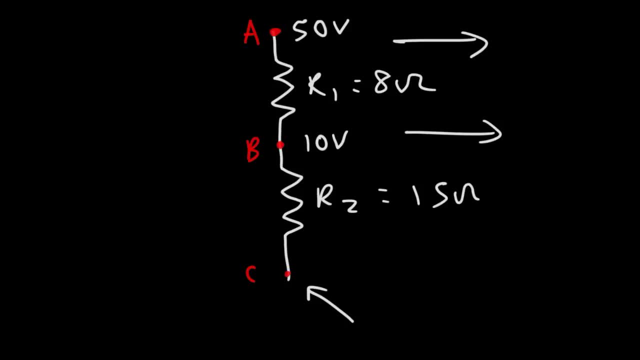 It's the potential difference between those two points. So it's 50 volts minus 10 volts, which is 40 volts. So that is the voltage across R1.. Now, in order to calculate the potential difference or the voltage drop across R2,. 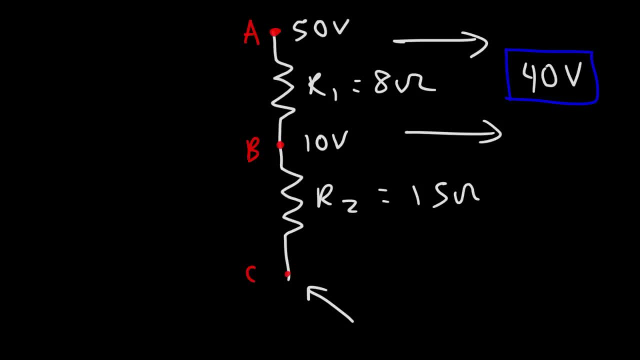 we need to determine the current flowing through R2.. Now, because there's only one path for the current to flow, we need to determine the current flowing through R2.. If current flows through R2, it's going to be the current flowing through R3.. 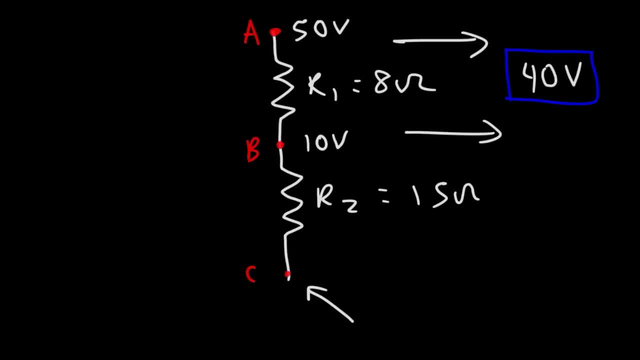 So we need to know the current flowing through R1.. So we need to calculate the current flowing through R1.. We'll call it I, So let's use Ohm's Law. V is equal to I times R, So V1 is going to be equal to I times R1.. 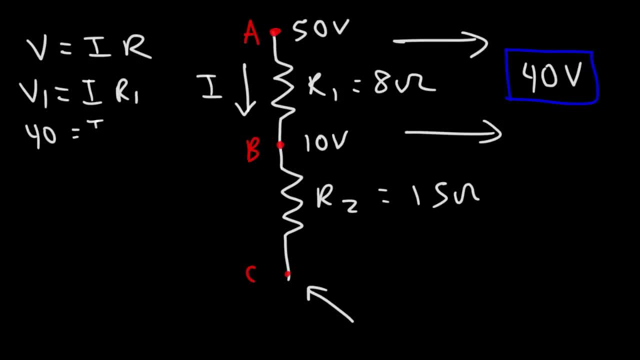 V1 is 40,, that's the voltage across R1. And R1 is 8. Dividing both sides by 8. The current is 26 volts is going to be 5 amps. So if 5 amps of current flows through R1, then the same amount of current.